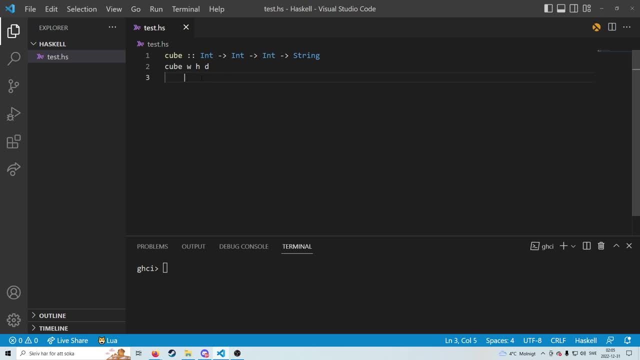 tab, and then we would do this large line here, And the way that guards work is basically that we have a condition, which can be true or false, And then we basically have- we have the return. So if this is true, then we return this, And the good thing with guards is that we can have 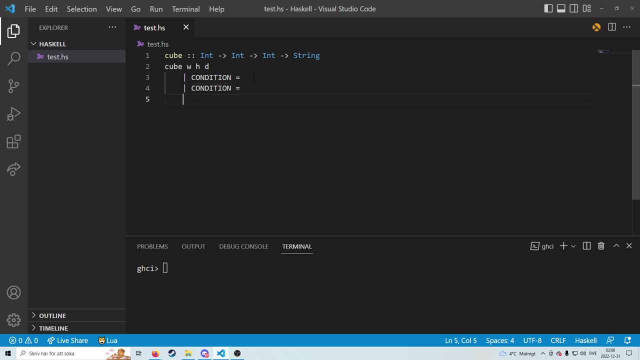 multiple of these. We could, in this case, have conditions followed by conditions, followed by conditions, And this is very useful in our case. So let's say that we first of all want to calculate the volume of our cube. We will basically just take width times, height times, depth. 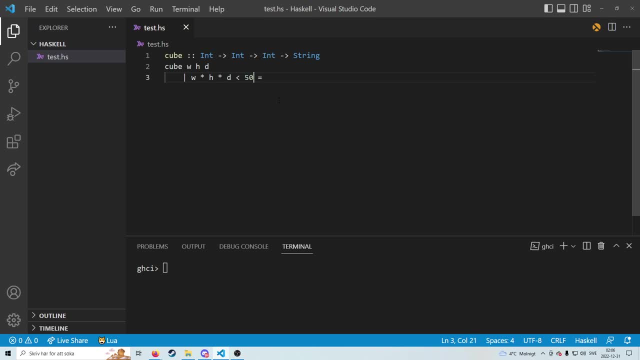 And let's say that if this is smaller than, let's say, 50.. And then we return small cube, And then we can do the same thing again. right, We can add another one And we can say that width times height, times depth, And if this is smaller than, 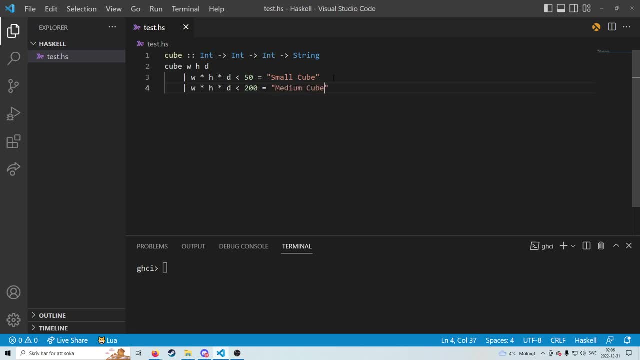 I don't know. let's say 200, we have a medium cube. And lastly, or let's also say that if the volume is smaller than 500, then we have a large cube, And then we can also say that we can also just have basically a base case. you can say: So we have otherwise here in the end. 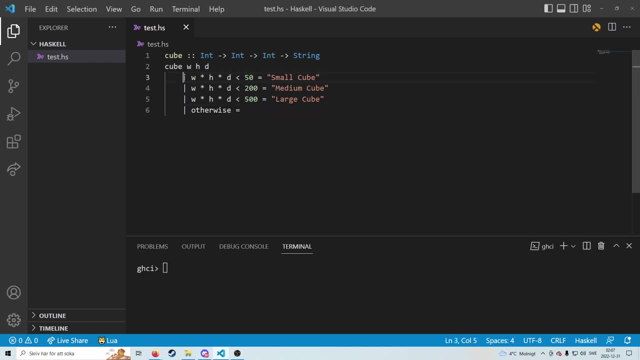 So if our function doesn't fall into these three guards, we basically have something that's larger than 500.. We can return enormous cube here, Even make it capital, Enormous cube, Make it real dramatic. Let's say that we were to try this function. 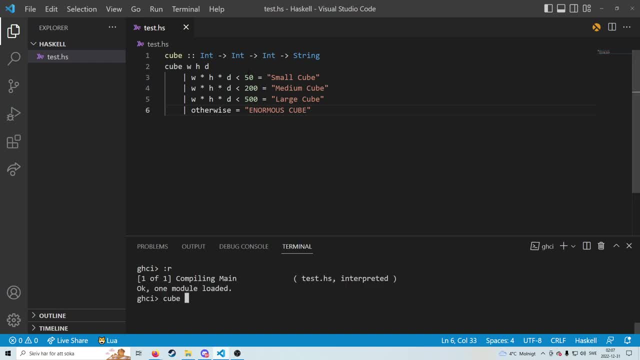 Let's say cube, where we have something which falls into that, the volume is lower than 50.. Let's do 345.. Oh, that's actually larger. Let's do 234.. Should be a small cube And, as you saw, 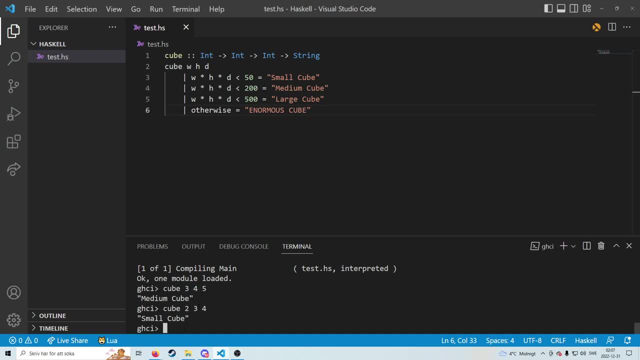 if I did 345, that would become a medium cube. And then we can. we can try something real big. Let's say 50,, 50,, 50 should be a huge cube And it returns an enormous cube. But let's actually say: 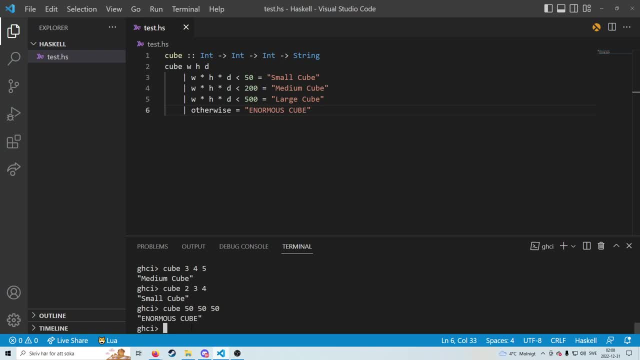 what if? what if I do cube in our case, and I actually send in a negative number, right It's. this shouldn't work in volume, because I can't have a side that has negative or basically a negative side. If I do this, I get the return small cube. So this is not good, right? So we can. 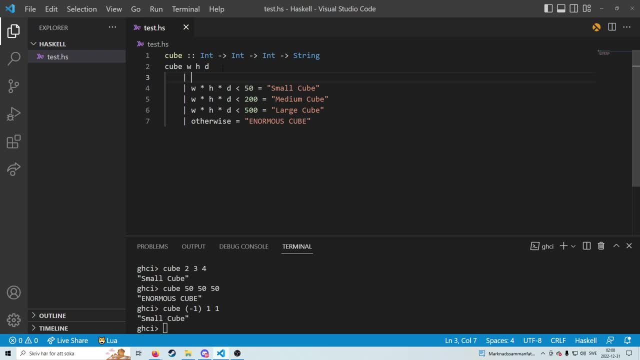 actually add another guard here. Oh, another guard. we can say that if width times, height, times depth is smaller than zero, then we return basically an error And we say a negative volume, which shouldn't be the case If we were to run this. 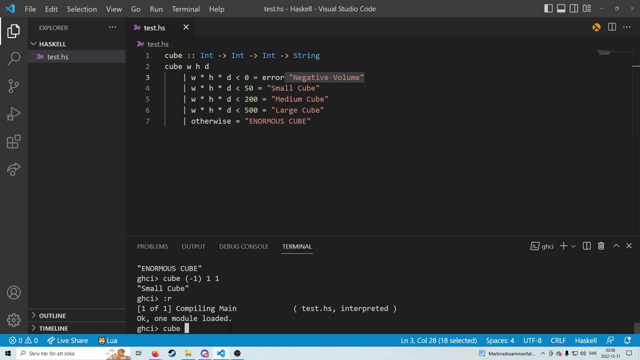 code, let's say cube, with, let's say, minus one, one on one, I would get an exception and an error, basically an error message which says that it has negative volume. But what happens if I make two of these negative? This would again oh, but this should also return. 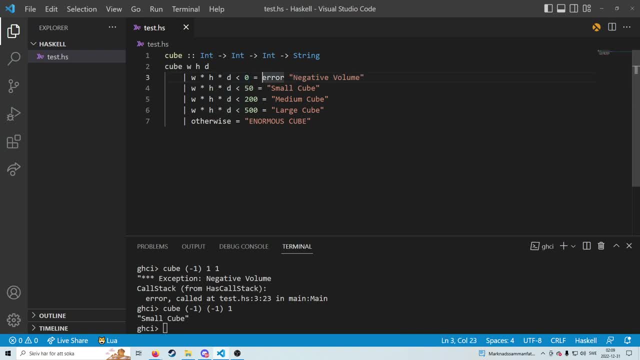 an error. So my, basically, my, basically, my guard here is wrong. So here I could actually add multiple. I could say that if one side is smaller than zero or another side- so let's say h is smaller than zero or d is smaller than zero- I return this error. Let's say that I were to 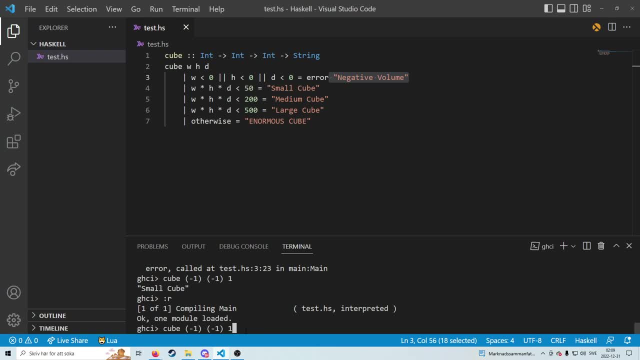 write this and do the same with two negative numbers again, I would get the exception error, error message again. But let's see our code here we have this calculation three times and this like, let's say, let's say that we had a very, a very, very complex calculation with like complex. 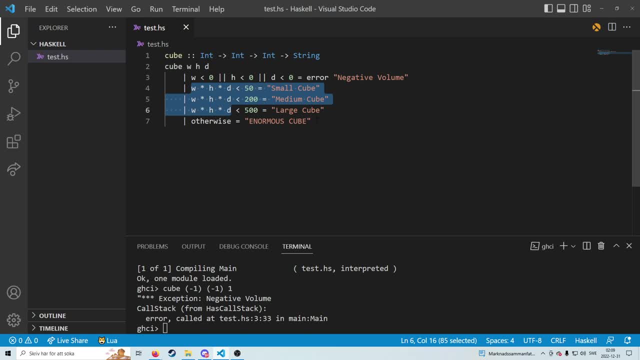 functions And then and then, to make our code look a bit more nice, we can use the the where So am here, Am here, I can basically define. So let's say I, I can basically define this calculation like I say that were volume is equal. 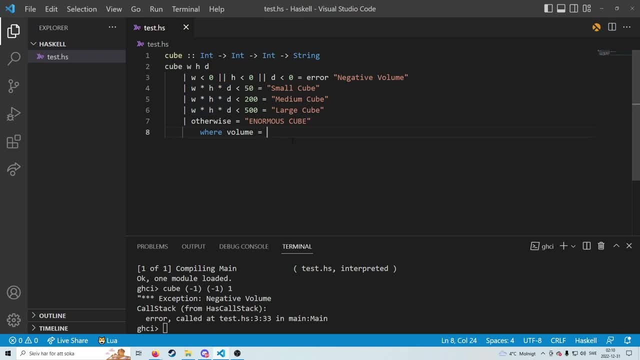 to, and then I can basically Just do this: I can take this calculation and say That volume volume in this function is basically equal to this calculation, And then I can take volume here And I can basically just paste this in here: Am.